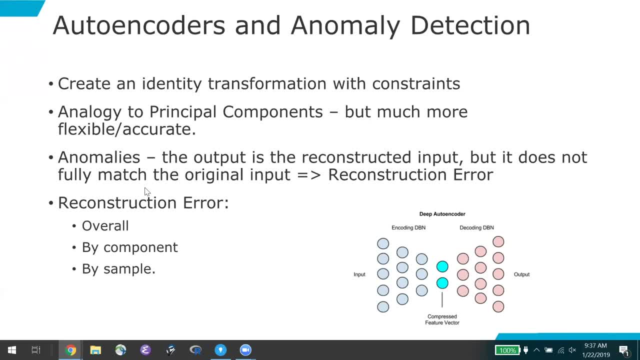 encode the information into a smaller number of nodes or features, which is very analogous to principal components, where you would normally take the largest few principal components and say that that's most of the variation in your data. So it's a very similar process. So we're going to 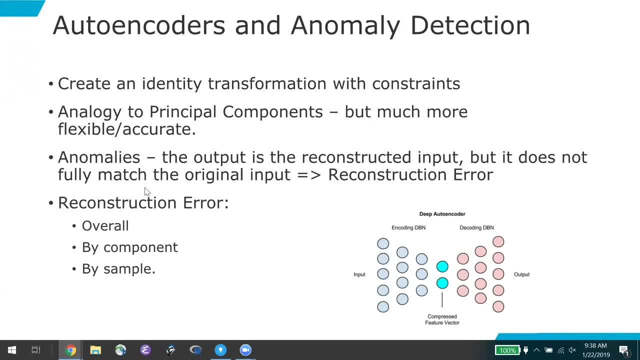 and then the smaller components are noise. But here what we're really doing is, you know, once we reproduce the input, we're looking for the mismatches, the imperfections in how that has been done, And that gives you a quantity that's called the reconstruction error. It 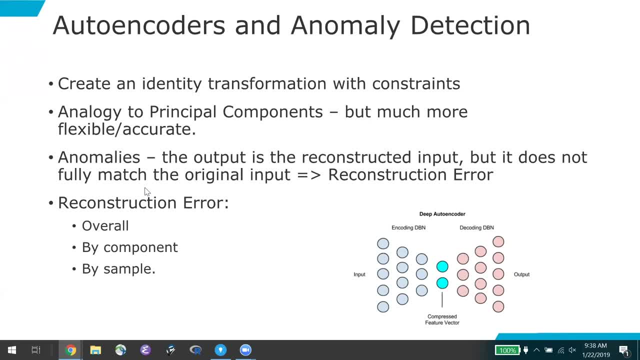 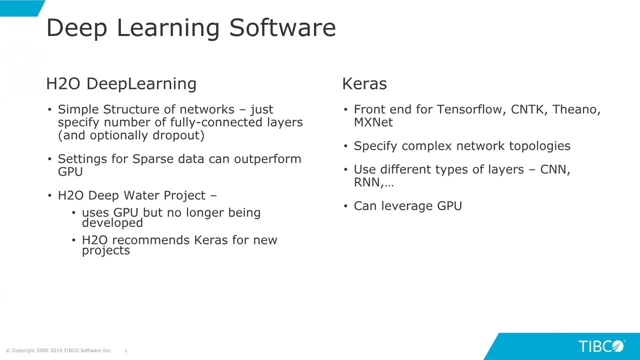 basically says how anomalous are these data points, And you can look at that by component or overall or by sample. Just a quick look at some of the tools that are out there for doing that: We in this DXP Spotfire template, we're using H2O deep learning, which is very approachable It. 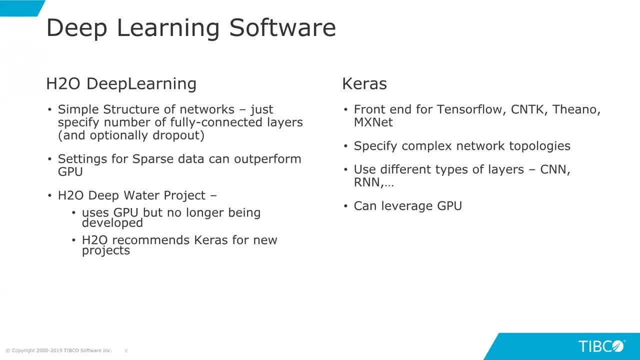 enables you to just stack layers, So it's fairly simple And there's just a few choices for the type of layers that you have. One of the advantages of the other family on the right under Keras is that it can leverage the GPU very well. I've grouped these together because Keras is one package that enables you to use. 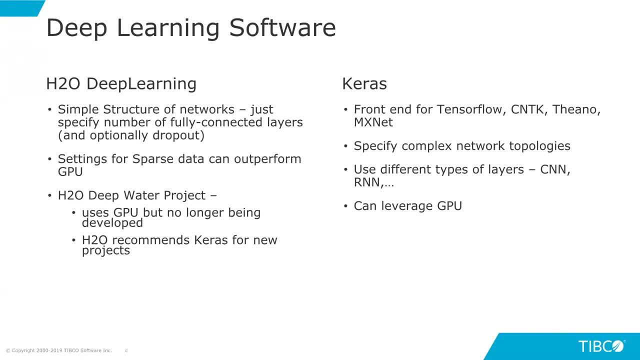 the same front end, And then, for performance purposes, you might use different, different systems on the back end, And all of all of those on the right have the advantage not only of the GPU, but you can specify more complex network topologies. but the learning curve is a little steeper. 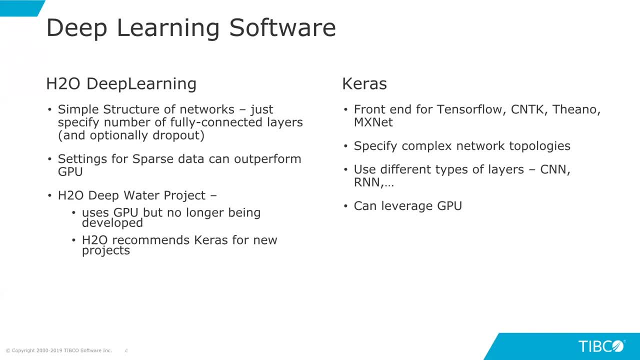 One thing that H2O does very nicely is work with sparse data, which, if you're working with text data, for example, it's very sparse And actually GPU doesn't doesn't work as well as as the H2O. I also just very briefly mentioned a deep water project which you might hear about, but it's it's mostly been. 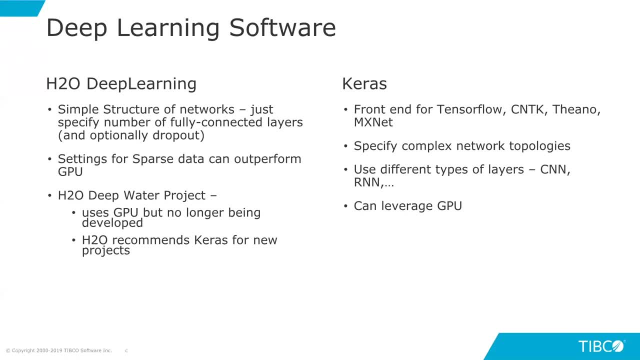 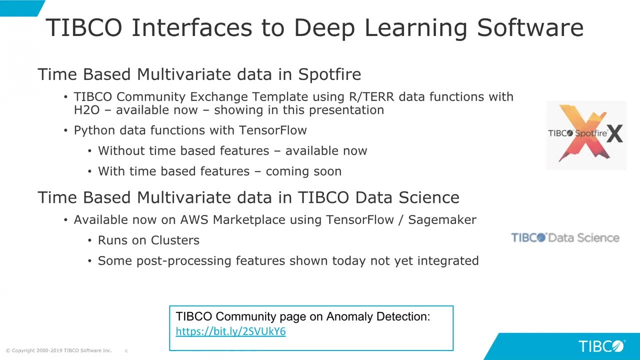 abandoned in favor of Keras for that type of problem. So TIBCO has looked at a lot of these and created demos and accelerators using different TIBCO products. So TIBCO has looked at a lot of these and created demos and accelerators using different TIBCO products. 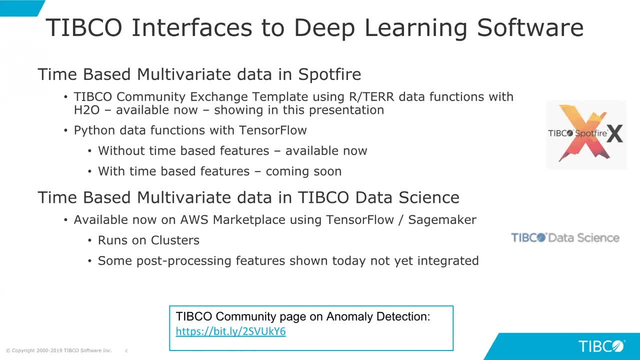 So TIBCO has looked at a lot of these and created demos and accelerators using different TIBCO products products. The one we're going to show today is this first one, and its strength is its very complete ability to do post-processing in a graphical way. There's also a Python-based 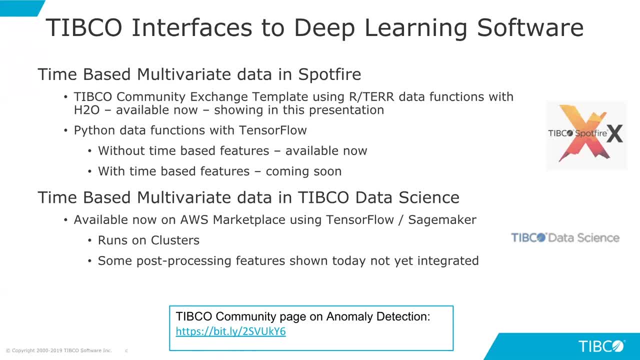 demo in Spotfire using the Python data function and also using TensorFlow. So you can also take a look at that on the community site. At the bottom you have a link to the community site with a single page that sends you to all our anomaly detection demos We also have 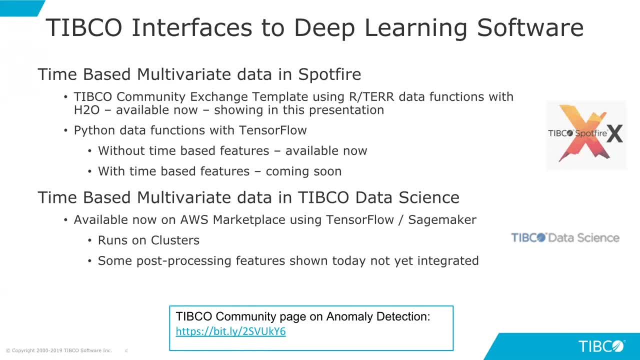 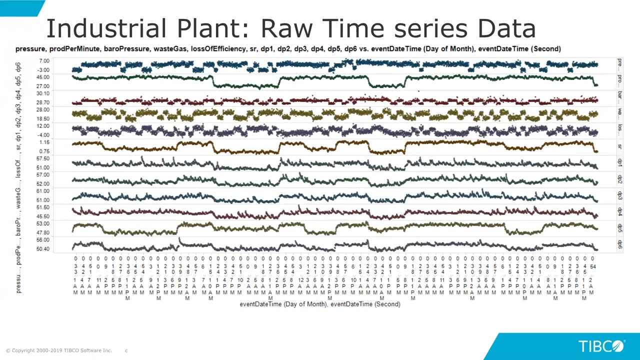 the AWS Marketplace offers one of our packages that uses TensorFlow in connection with SageMaker. It has the advantages, It's already set up to run on clusters and is definitely worth a look. So what is the problem? Let's look at the problem that we're trying to solve. We have a lot of time series from different 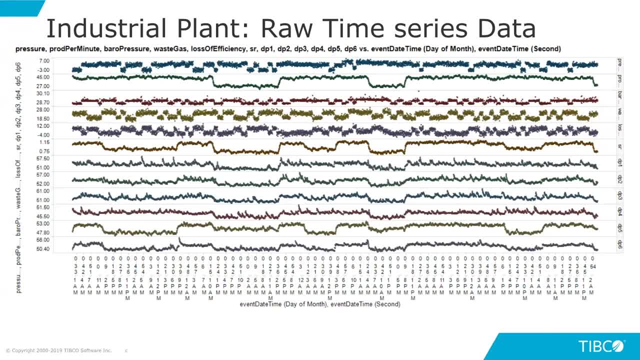 aspects of our process. Usually, I think of this as a factory with a lot of sensors. That's a good application, But anytime you have multivariate time series, you can use this kind of technique And again, unlike K-Means, the way Tomas presented this, is unsupervised. We don't necessarily have labels, or not very many labels. 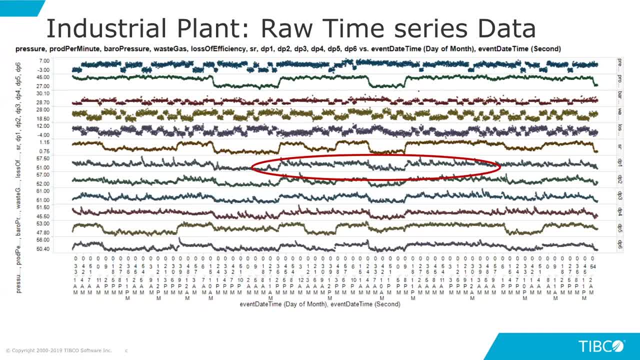 So the very traditional way is to look at one time series at a time and say, oh, this has gone out of the normal range by looking at the variance of what has come before. Here we take a cross-sectional approach. So for the analysis that we do, we have these vectors corresponding to individual points and then the very important time dimension is added in the post-processing and you'll see how that's done. 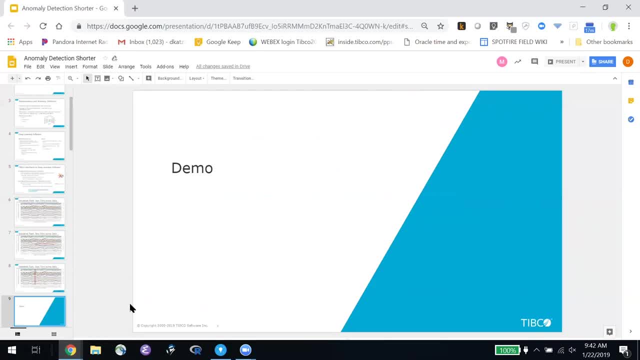 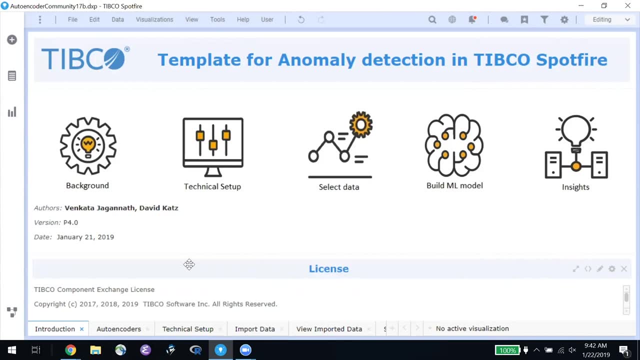 So let me switch over to the live demo, and this is what you'll see if you download the demo from the community site or the template from the community site, and it's showing here in Spotfire 10.. You can also use it in earlier versions of Spotfire. It'll look a little different. As you can see, Spotfire 10 has the pages or tabs along the bottom. 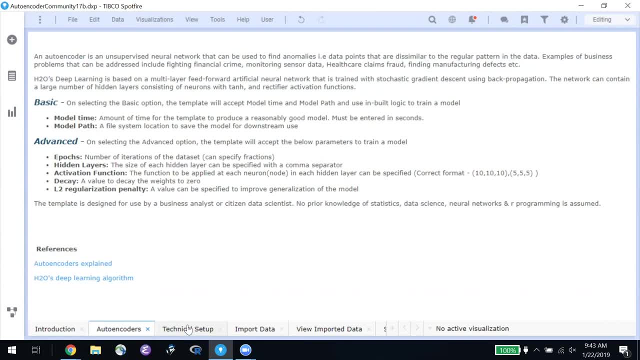 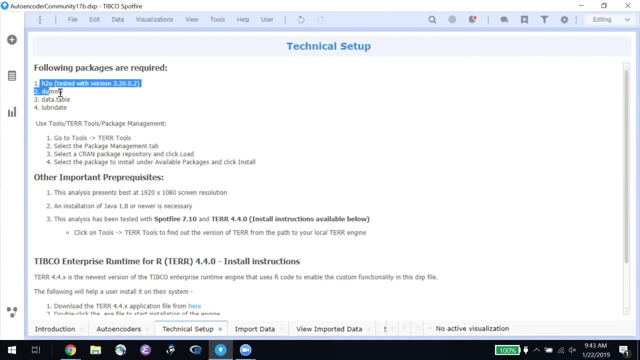 You've got the Just a little introductory information about autoencoders, and then the setup is actually pretty simple. You just have to make sure that these packages are available to R, And so what you do is go to tools, which I can't see because Zoom is on top of me. We go to tools, care tools. 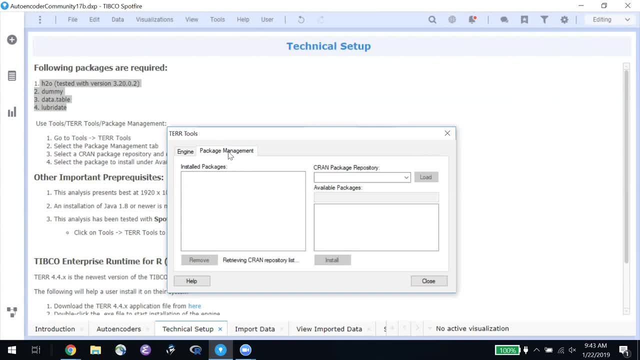 And then we go to tools care tools, And then we go to tools care tools, And this enables us to go to package management, and what it does is it retrieves what is already installed and also gives you this list, but I always just use the default. 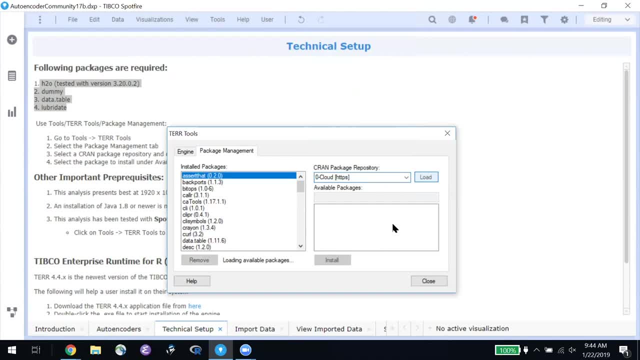 It's not really necessary to localize for most of us, although sometimes that gives you better performance. And then you have all the packages that are available. You have a search bar and you just need to go through these four and install each one of them. 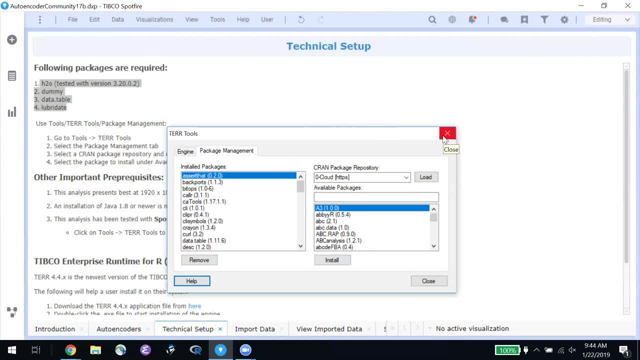 And then you have all the packages that are available. You have a search bar and you just need to go through these four and install each one of them. So that's already been done, but I just wanted to show you that to make your path easier when you go to try this yourself. 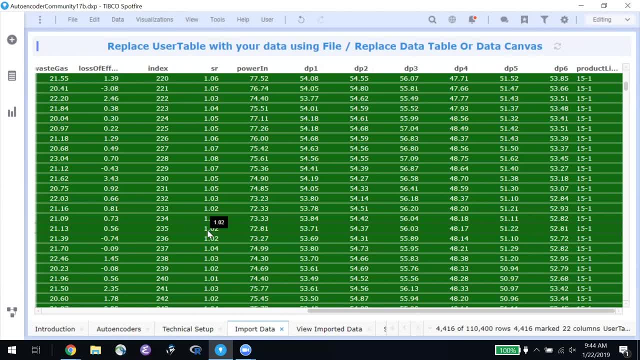 The next step is to import your own data. Now I've got sample data in here and you might want to take a look at that, but most of you will be most interested in loading in your own data, and that's done with replace data table. 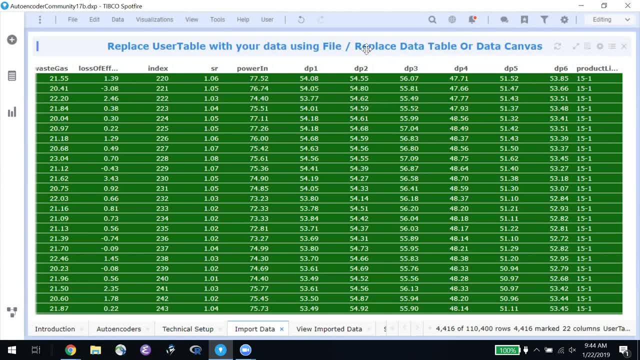 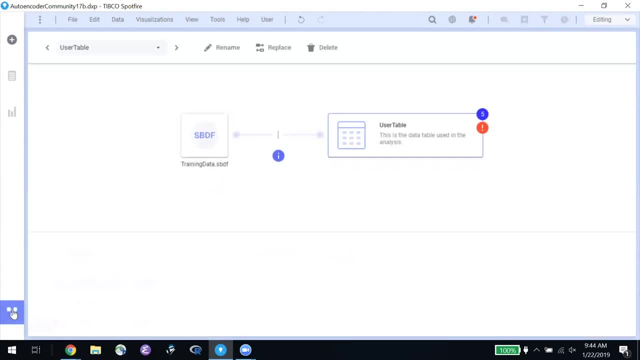 Now in previous versions of Spotfire. that's just a menu option: file replace data table. Right now it's part of this data canvas which Michael showed before, but it's got you know all the tables available and the ability to replace one of them here. So 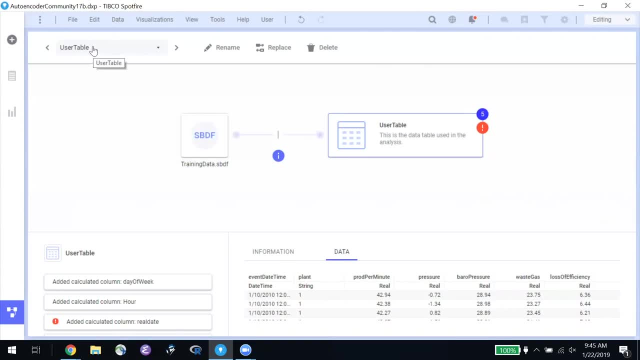 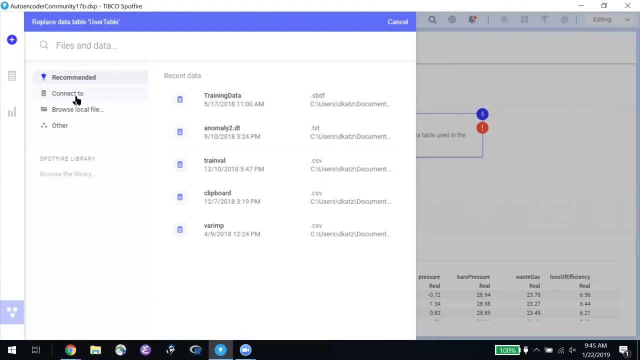 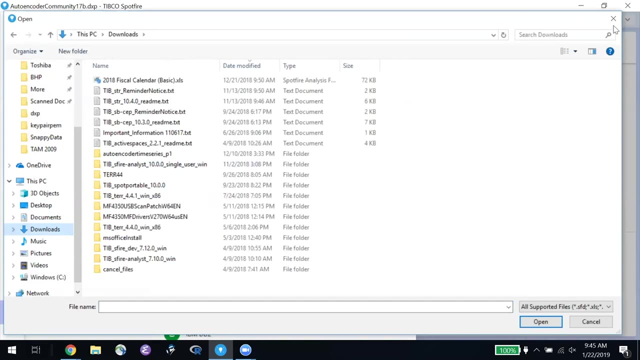 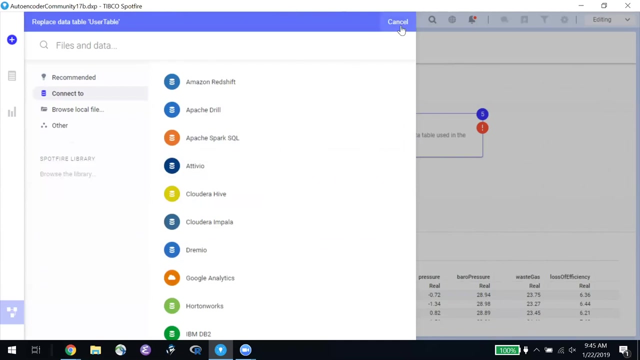 what the user table is, the one where you would replace it in order to use it. So you can use your own, your own data, and when you choose that, of course you get you know, database connections or you've got local files that you can look at. So any tabular data can come in here, either through one of these connectors or as a local file. And once you've done that, 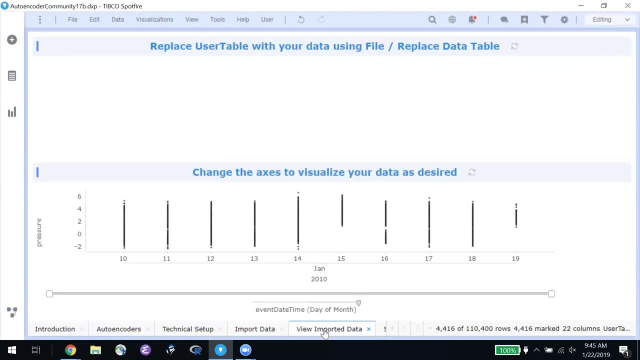 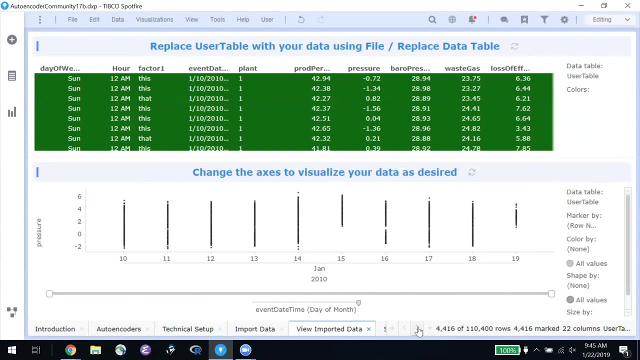 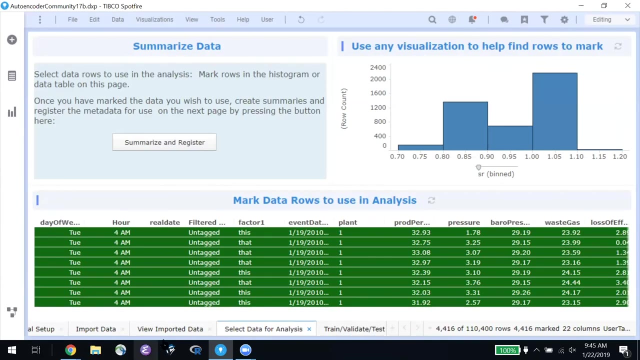 we close up the canvas and we'll take a look at that data. This page is really here for free exploration of the data with any of Spotfire's visualization or analytics tools, But then we get more focused on selecting data for the analysis. we want to want to do So here by a marking. I've selected a slice of data that represents one factory and one product. 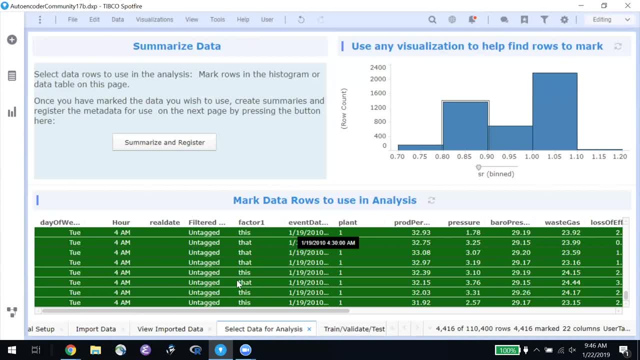 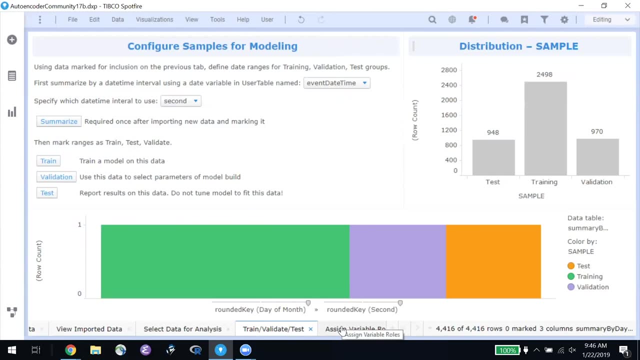 And that's it That helps in our time series if it makes sense to look at those one one at a time. So then we register that data- basically use this button here to ingest the data. And then there's the step where we define three samples. So, like in many 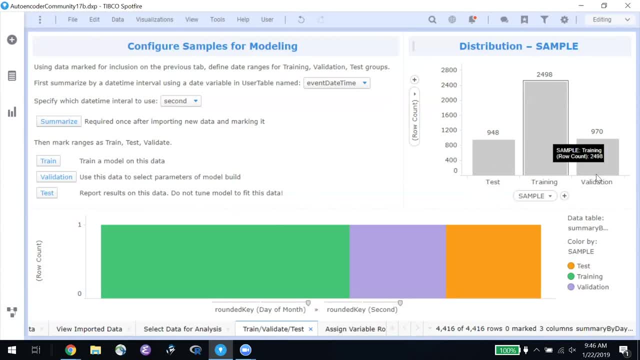 data analysis tasks. we have a training data, we have a validation sample and a test sample. Here we do something just a little bit different in that we do it in a time-based manner. So, in order to start fresh with the new data that we've 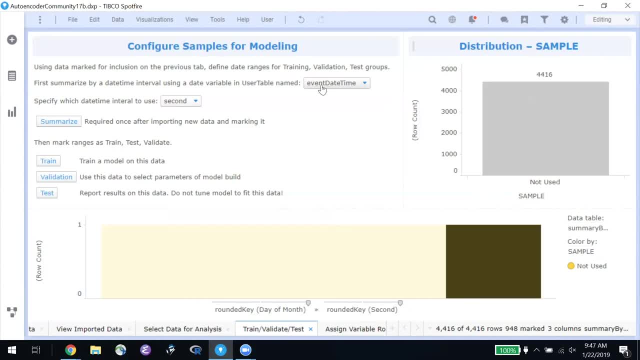 put in. we summarize using the time column, the date time column that we select. If there are multiple ones, there'll be a drop-down Here. in this case, we just had the one, And then we do this based on time intervals. The reason: 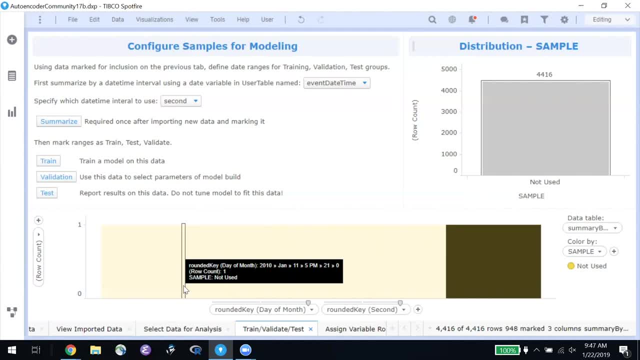 for that is to prevent overfitting. If you did a random sample, then anomalies in the training sample and the test sample, the validation sample, they'd all show up pretty much as normal elements of this data. But if you want it to generalize from a training sample which you can identify this way and then 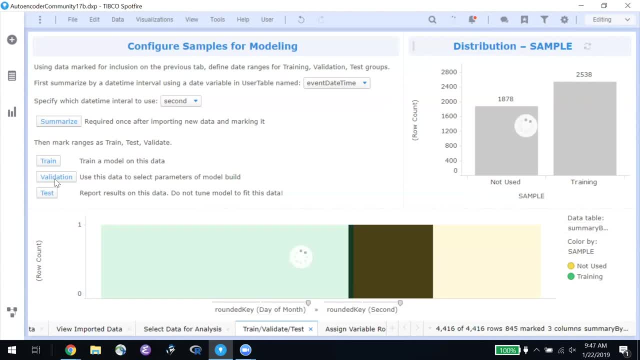 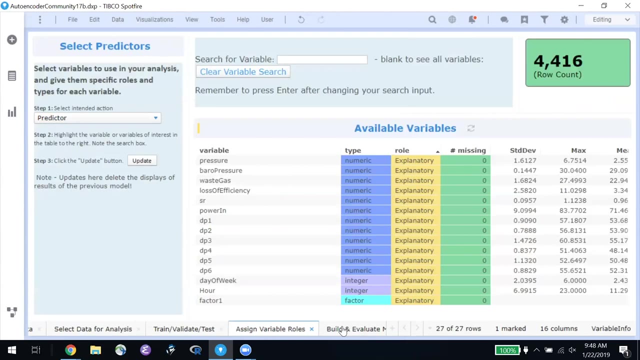 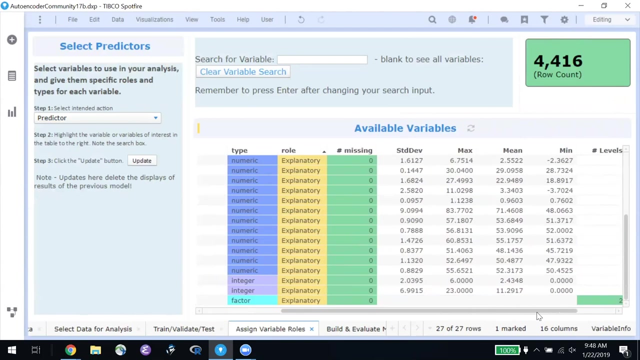 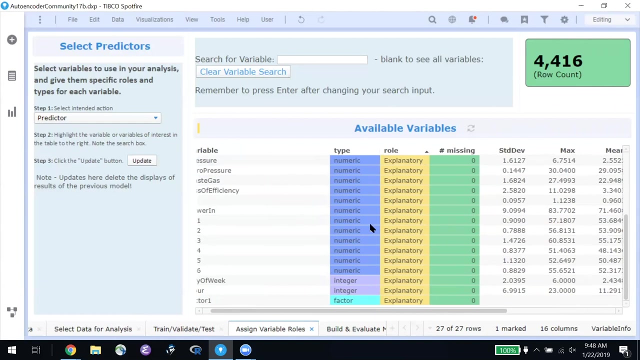 just by marking you can identify a validation sample and optionally you can have a test sample as well. that actually works better with this kind of time series analysis for anomaly detection. Then we have whatever data that you've ingested and marked For analysis, we get a nice summary of them and we have the ability to include. 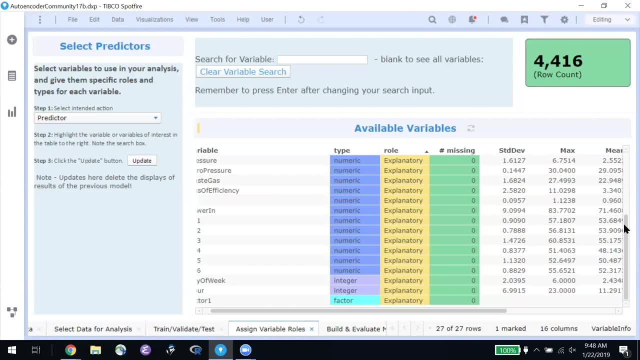 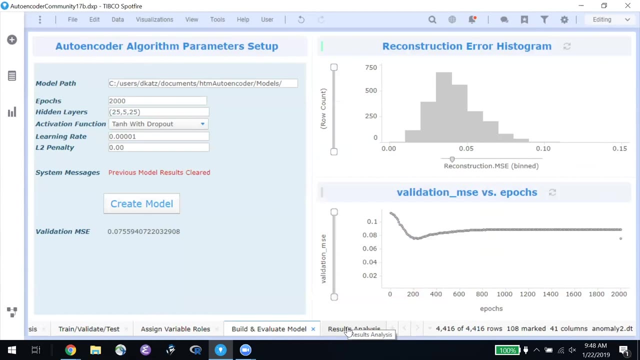 or exclude them, Or in some cases we would change the, the data type, and that's done with this interface here. It's very straightforward to use. And then we'd like to actually go and build a model and that we have a number of. 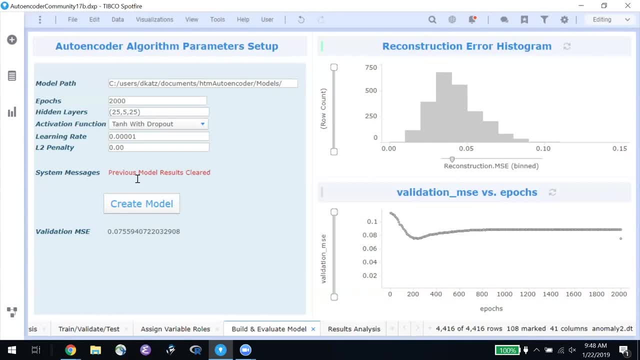 basic parameters that control the building of the model. So the model path is simply where you would write the output to save it for later. The epochs are: you know how long do you train, how many times do you go through the data in your training process And the hidden layers? this is the way. H2O2,. 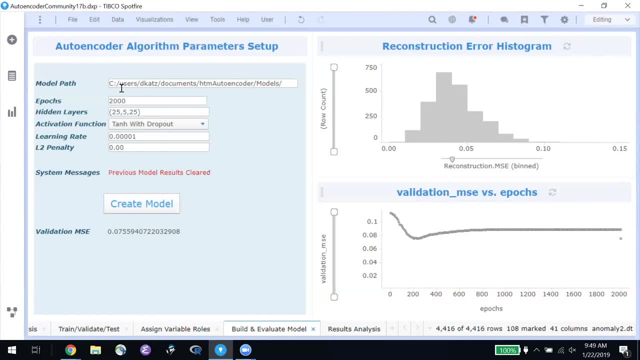 H2O looks for your stack of layers. So we've got 25 input layers and five hidden. you know, five constriction type hidden layer And then 25 back to restore or reconstruct the data And this reflects that sideways hourglass that we 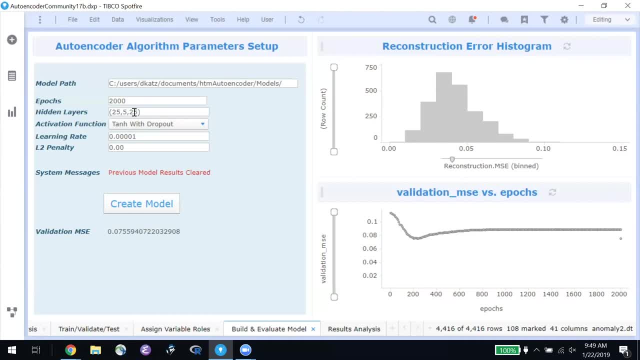 saw before, and you can put in any number of these layers. typically you want a number that's somewhat larger than than your actual inputs here. you know we've selected a dozen or so inputs, so we put in 25, and then I'd say mostly this, this: 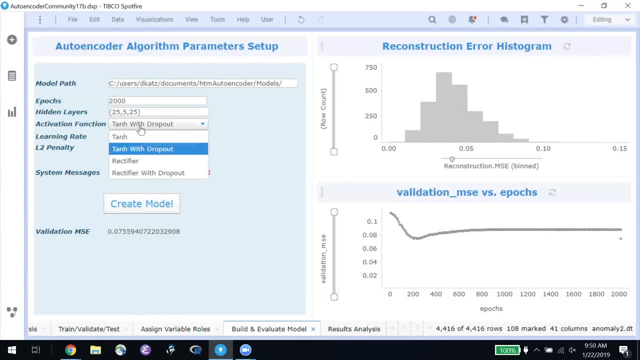 activation function is should be left at this setting. but you do have these different options of the technical side of building deep learning models, and the learning rate is a good one to adjust so that it's not too small, which would make things very slow, but if it's too large you tend to. 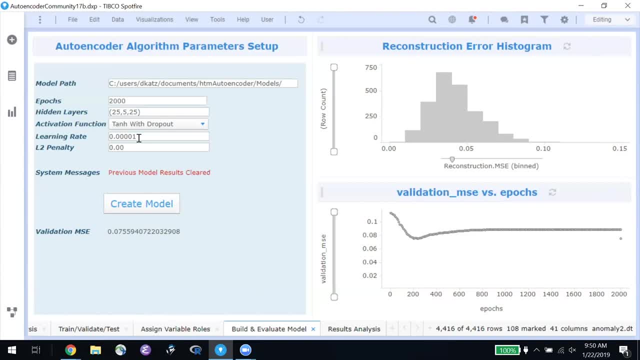 not get as good convergence as you would otherwise. so here you can create the model and you have a couple of diagnostic plots which can be very useful. this is validation error plotted against your the amount of training you've done, and that's extremely important. what you want to see is this kind of pattern where 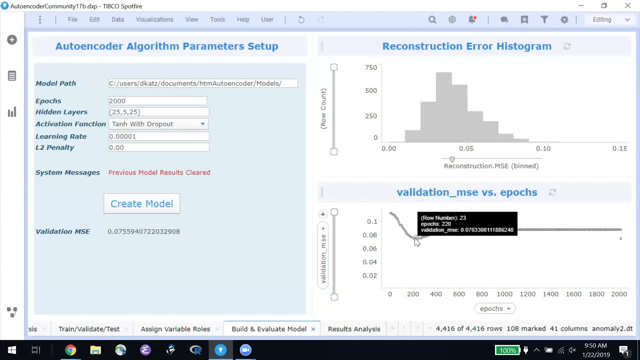 you. you get a tighter and tighter fit, but eventually you get overfitting, so the error increases. h2o is very nice. it will remember your minimum and use that for the subsequent calculations. now we talked about the reconstruction error, so here's a distribution bar chart of the 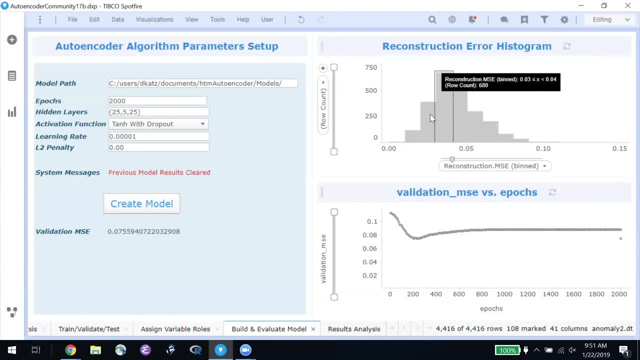 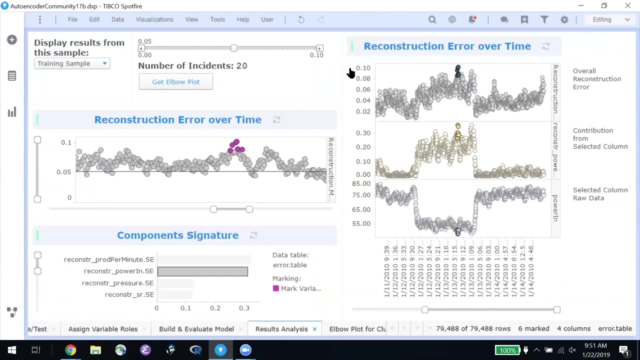 reconstruction error and we see that mostly you have a small reconstruction error, but at a certain point there are a number of cases which are potentially anomalies because we can't reconstruct them very well. so now we look at this in a time series context. so here is our training sample and we also can look at the 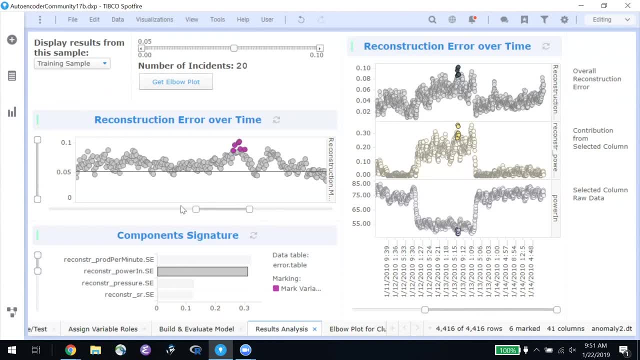 validation and test, and we have these sliders so you can look at it. this is the thing that I found really interesting about this is that in most cases, you don't have isolated points in time where there's a problem or an anomaly. the anomaly tends to build up and last. 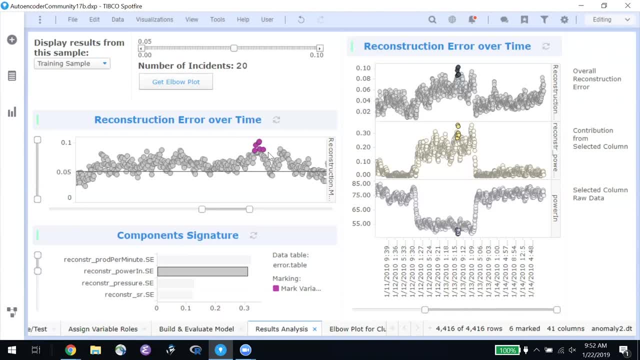 for a while and and then resolve either by intervention or for some other reason. So I like to think of these as incidents. So if I mark this incident here, I get the variable importance which is actually the contribution to the reconstruction error by each of your input variables. 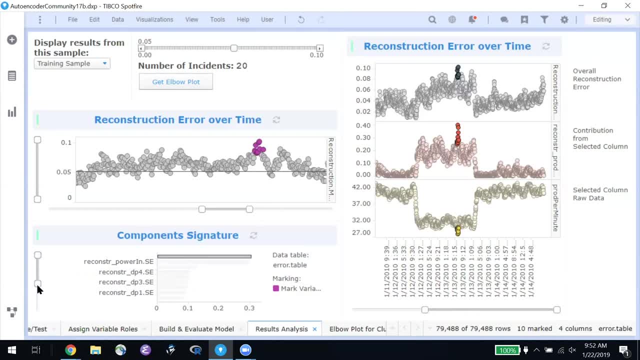 So here we see. you know, even though there are a lot of variables, the ones that really contribute a lot to this particular incident are these top two or three, And by selecting this we can get time series broken down to either the raw data.